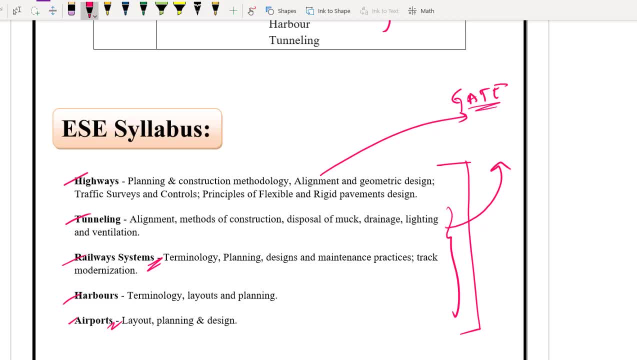 just given like one or two words, like direct question type: dedhi hai, What is the runway length, What is the exit way length, like that? So obviously the gate syllabus is going to be very much easier compared to ESC when it comes to transportation engineering. So the syllabus is very much in detail, But the rest, the topics are very few. They give directly like one or two words, like direct question type: dedhi hai, What is the layout of the train? What is the layout of the train? What do the trains have? What is the layout of? 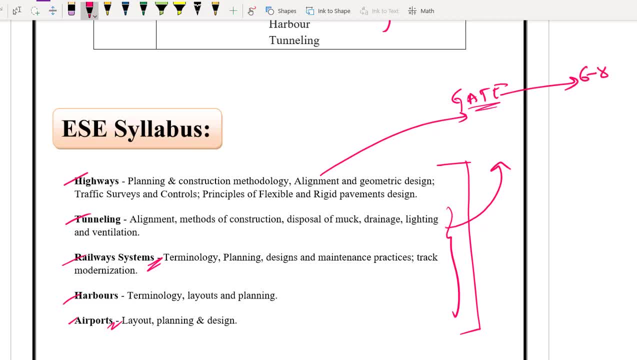 space. Let's do the whole process. So if we are talking about the layout of the train, then there will be 8 marks in transportation engineering. But if I'm talking, if I have to talk about weightage in gate, every year you will be getting 6 to 8 marks from transportation. 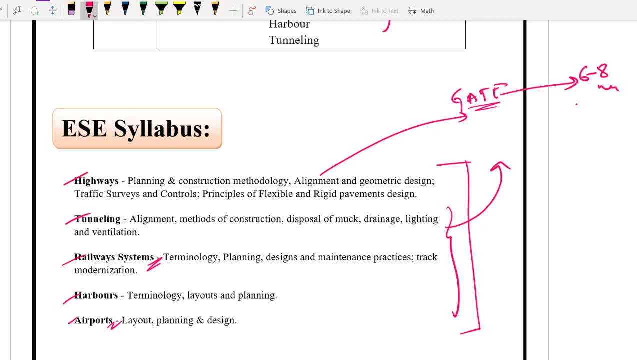 engineering Out of this. if you are taking, let us say, 8 marks, Okay, In a year you got 8 marks from this transportation engineering. at least 5 marks will be from highway and the remaining 3 marks it will be from railway and airport. ya, Now, highway should be your. 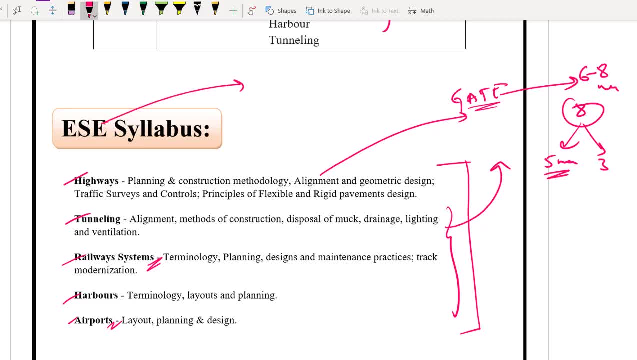 first priority if you're preparing for gate. And now, when it comes to ESC weightage, the weightage of ESC is not uniform. What is the weightage of ESC? It is not uniform Sometimes. Sometimes he can ask you only five questions and sometimes he will be asking you 11 questions. 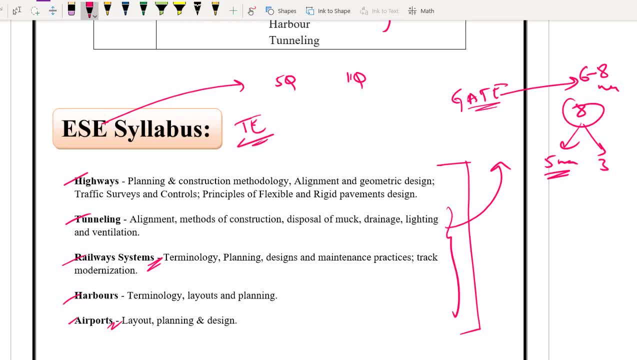 But on average, the weightage of transportation engineering is unfortunately less compared to other subjects, which is actually good, also Okay, Because there are subjects like building materials, or it could be environmental or soil mechanics, which have a decent weightage, but the transportation engineering doesn't have a huge weightage. 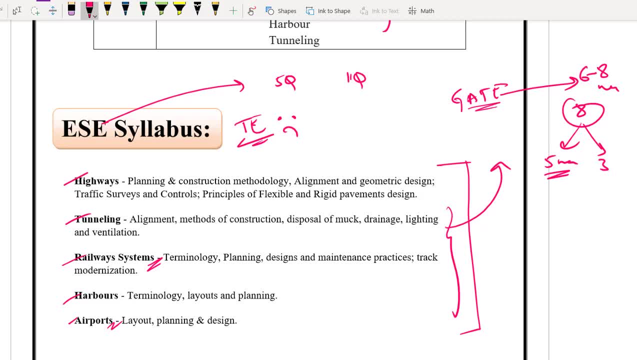 in ESC The weightage is very less. If you are getting like 10 to 11 questions, you will be lucky, Okay. If you are getting like 10 to 11 questions, hardly 10 to 11 questions will be coming in. 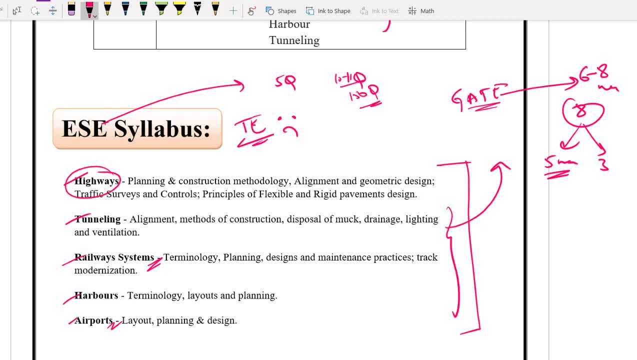 your ESC Out of it again. majority will be from highway only. If there are like 10 questions, 6 questions, 5 or 6 questions will be easily from highway and the rest 4 to 5 questions will be from the remaining topics, like airport railways. 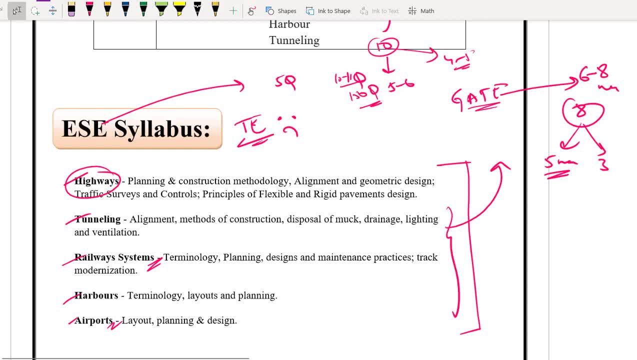 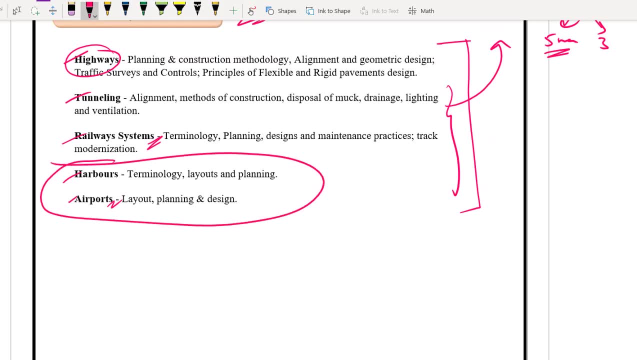 and so on. Okay, I hope it is very clear Right Now. let us continue with the very first topic. Actually, I got a lot of requests from the students. sir, in our coaching centers they don't teach us airports and harbors. topic: 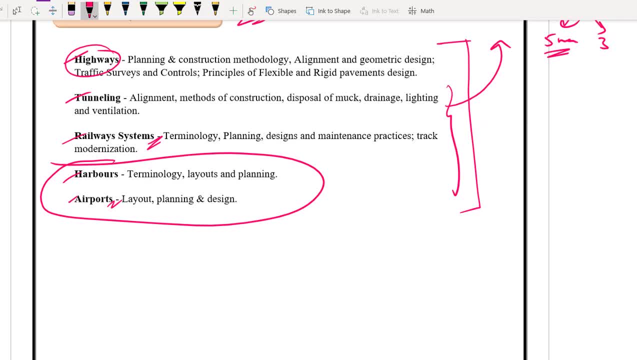 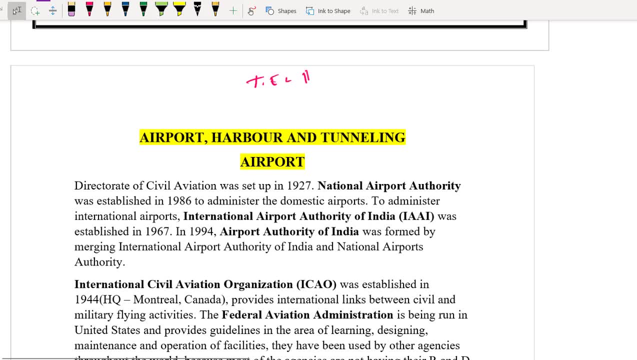 Can you please teach that to us? in the beginning I said I agreed Okay To their request And I'm starting with airport now. Okay, Transportation engineering two, and this will be the module one, and in module one I'm going. 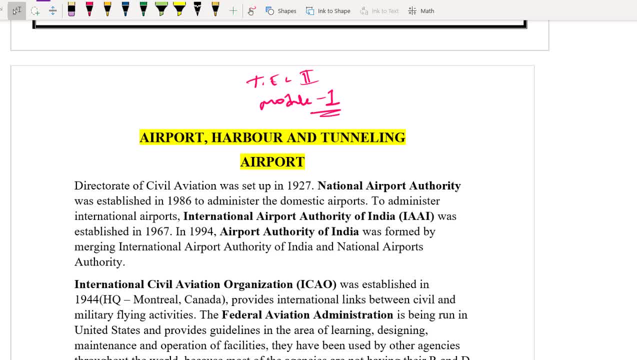 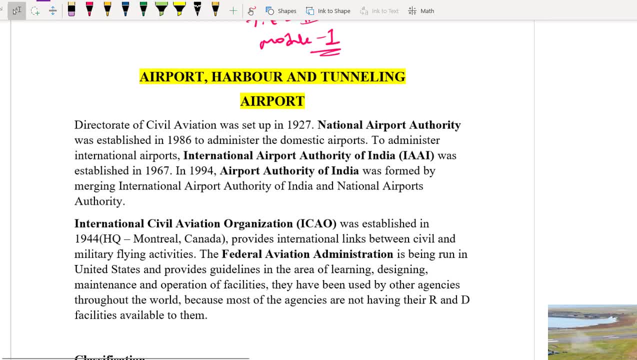 to start airport. Okay, First we'll be finishing transportation two and then we'll jump into transportation engineering one. Now, when I'm talking about airport, you should have a basic knowledge of history about Indian airways, because because in small examination you can have a direct bit related to that. 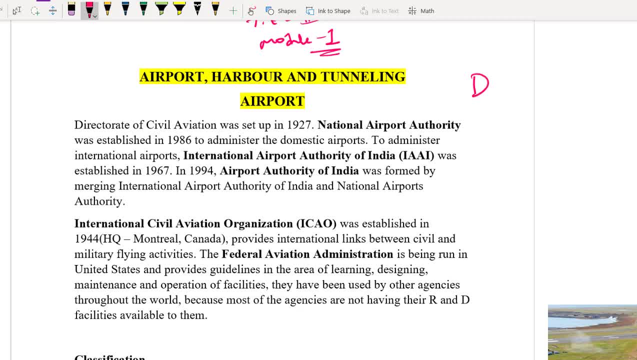 Okay, In India there was a department related to aviation established in 1927, and it was called as direct rate of civil aviation. Okay, 1927, during the British Raj, only we had this direct rate of civil aviation Okay. 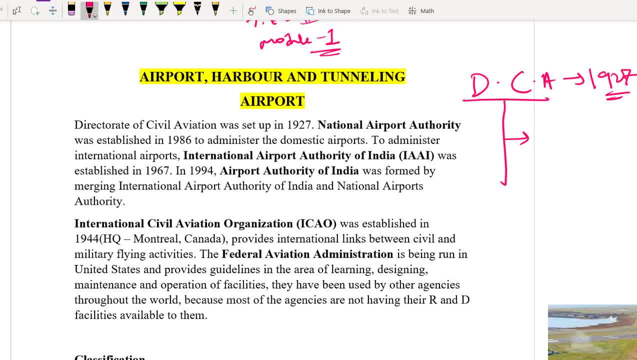 After that, after a lot of years, we felt that there should be a separate department to handle international traffic. That's why, in 1967, we had IAAI. What is the full form? International traffic, International traffic- Okay. 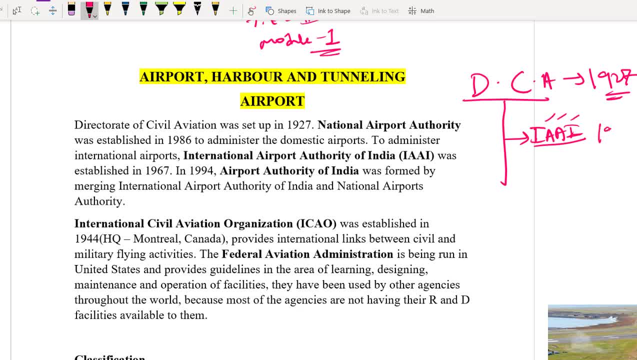 And now we are in показ Nakosa foreign airport authority of India, and it was established in 1967.. Sometimes, yes, also place a crucial role. Joe did short exams online Kali. I asked: ah, already it, Ken. that's why focusing 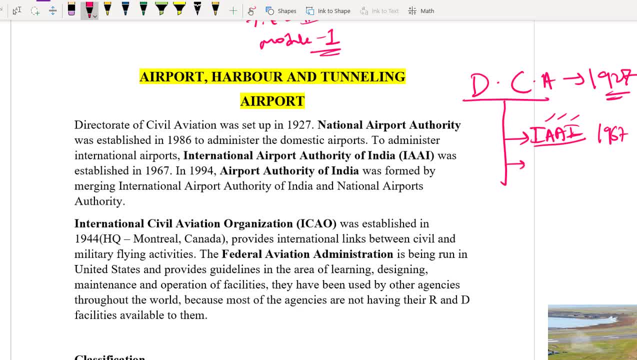 Okay. After that they feel like: okay, domestic flight frequencies, well increasing. That's why we have to establish one more department. So they have started National Airport Authority, NAAM. yeah, Court authority in 1986.. Okay, after that. 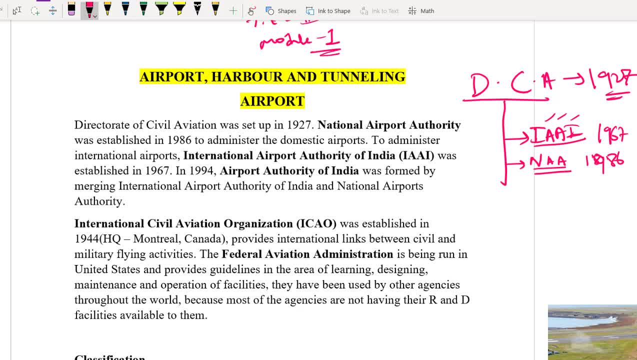 And then they failed. Why do we need two different trips? Yeah things, can we merge it? and finally, we got airport authority of India, which we currently have. almost every year there will be a notification of a AI. if you don't know, just google it apply. galena saw those on okriyanto herself, nickel. 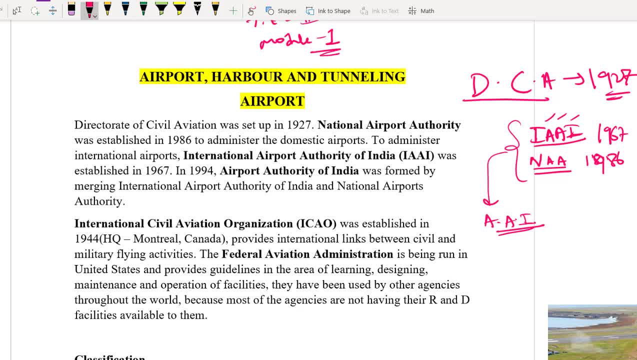 day. okay, there will be vacancies of civil engineers also. okay, because airport banana Mitch, I can China maintenance kill a bitch a. so have a look on airport authority of India website also. now, this airport authority of India, whatever was established that, it came in 1994. from now, from that time, 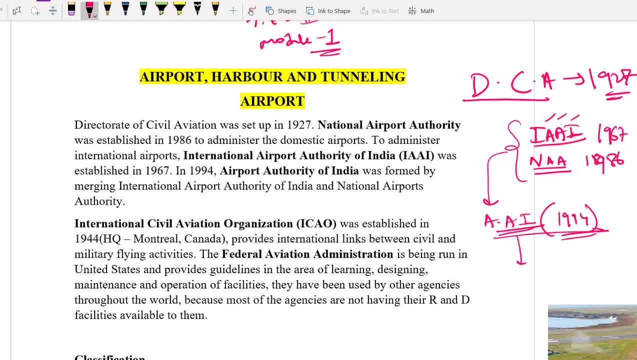 we are using the same thing. okay, airport authority of India regulates everything related to airports and aeroplanes in India. I hope it is very clear for you. similar to that, obviously there should be one international organization guiding all the countries right, because India get flights, India they hang on. 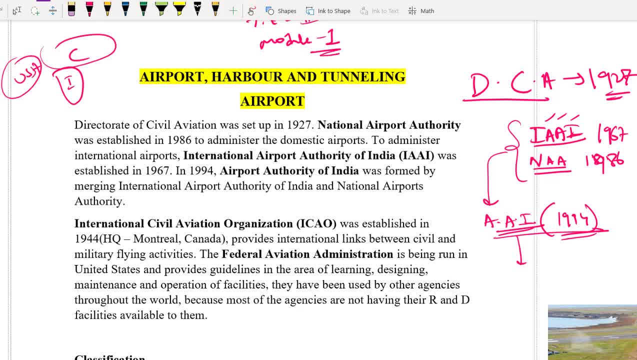 China get flat. China, they hang on. USA k flights- USA, they hang on. but to provide the guidelines to all this country, to set the regulation, there should be some organization. that organization is in Montreal, Montreal camp, a Canada pair. okay, North America. may North America continent my Canada. 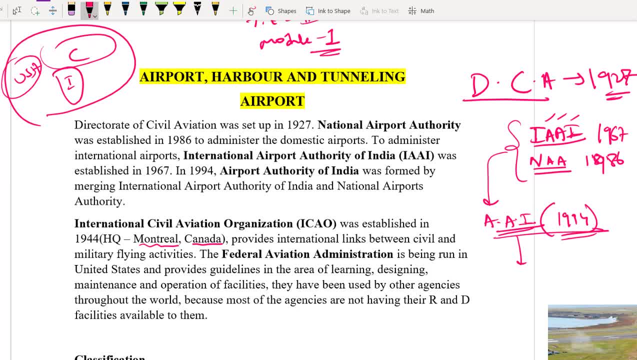 country, a Canada country, me, Montreal, XT a and the headquarters of international civil aviation organization. I see a. oh, he is present in Montreal. it could be asked in like paper one. general knowledge subject of your state, PSC varies. I see a. or located answer: Montreal, Canada ticket. so 1944 may form, oh gata, international. 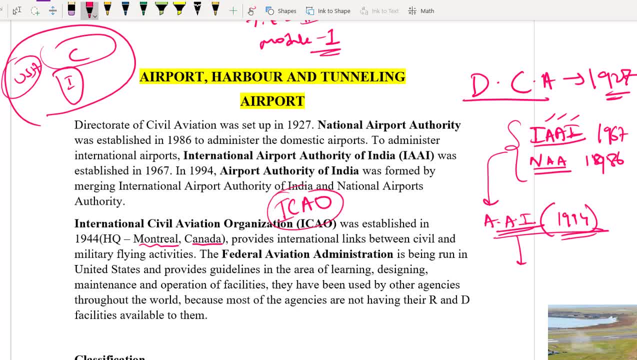 civil aviation organization and it is in Montreal, Canada, and all the rules and regulations, basically job a related to airport and aircrafts. it is given by- I see a who now in ICU. there is one very major role-playing organization which is FAA- FAA, Federal Aviation Administration of USA. they say India Kai AI Airport. 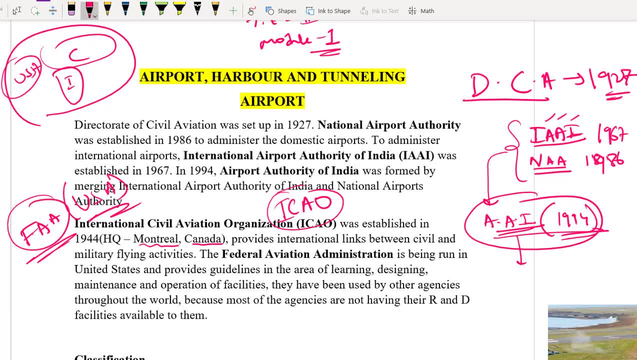 Authority of India. we have FAA and USA Federal Aviation Administration and it is super duper powerful. okay, whatever it says, mostly I see you will agree with it because they have a very good research and development wing. okay, oh just, and that's the telecoffee standard, right? i, because you will say the standards are really strong and good. 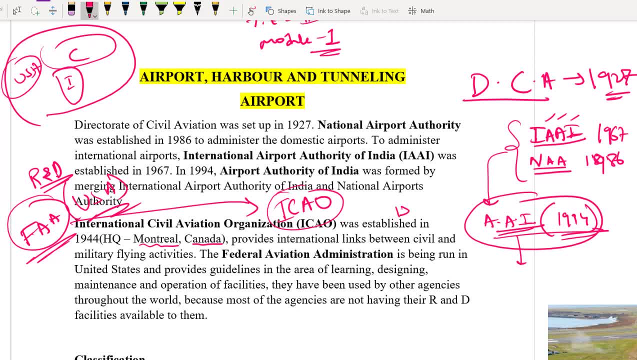 even the is course. whatever we are using in India- see the IS course- whatever we use in India, it could be related to steel, it could be related to concrete 99 percent. they are copy of US standards. okay, same to same: raga. we take that and we will talk about that, but we are not going to talk about that until now. so that makes sense. 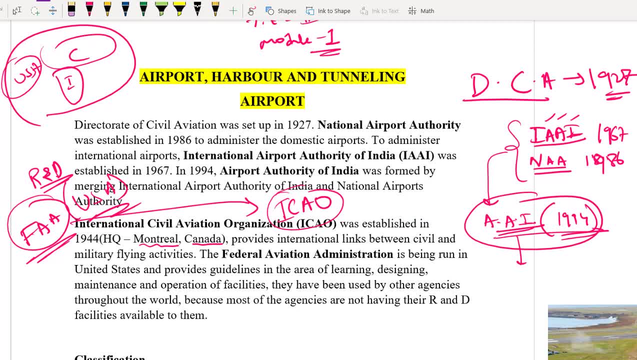 and just name it as IS code. if the units are different, we will be converting the units and then writing it as IS code. that's all we do. okay, most of the research is done by USA and after they do the considerable amount of research, they will be giving these regulations and, basically, ICAO will 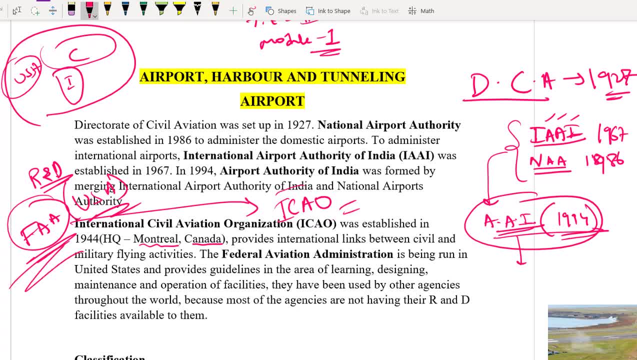 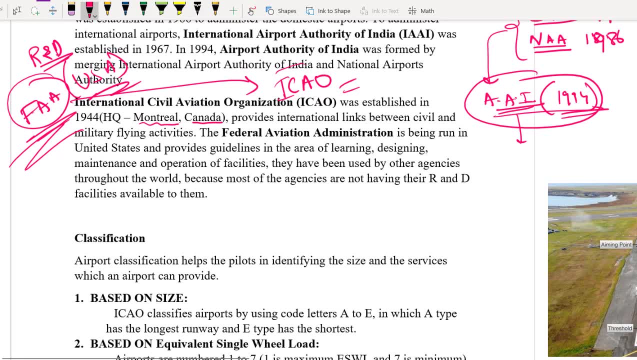 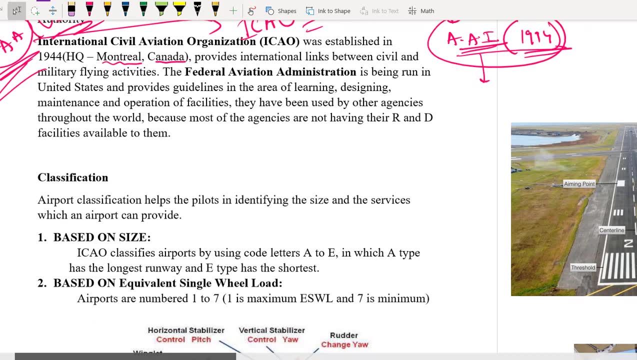 be accepting that and entire world will be looking forward for these rules and regulations of FAA, even including India. okay, I hope it is very clear. right, they are the strongest and we basically follow them. now, coming to the classification of airports. we have different types of airport based on the size or based on equivalent single wheel load. we are classifying our airports first. 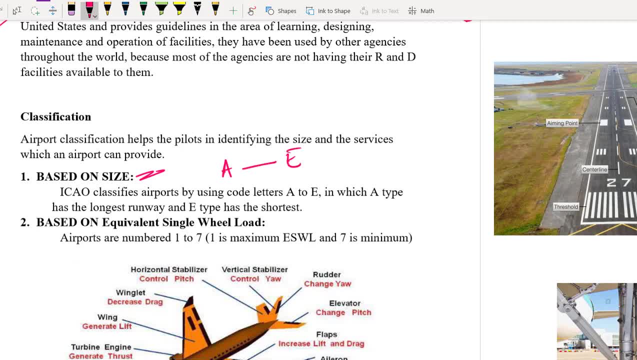 of all, based on the size. we can classify it from A to E. okay, class A airports. class B airports. class C airports. class D airports. class E airports. this is based on runway size. remember, this is based on runway size. that means A is the best one, which will will be having the 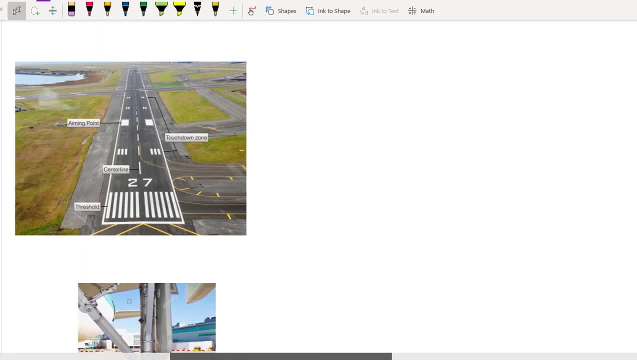 longest runway. what is runway, runway, what is the same how it is running, that plane will take offs off and land, okay. so A is the longest. thats why it is safest. also, if you have something long runway, it is good for you, right? so A is the best. then we have BB will be. 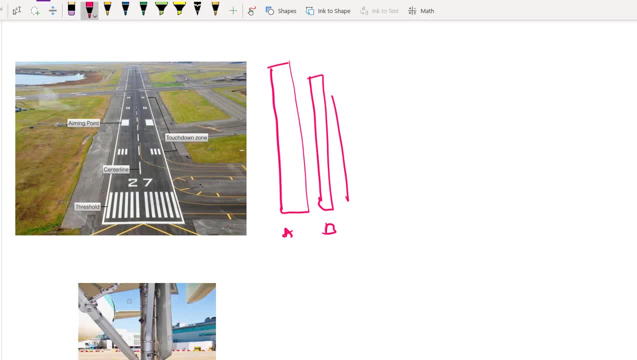 obviously shorter compared to A. and then we have CC will be obviously shorter compared to that of B, B, D will be shorter compared to that of C and E will be the shortest. we have only from A to E and A is the shortest. sorry, A is the longest and E is the shortest. please lie down. 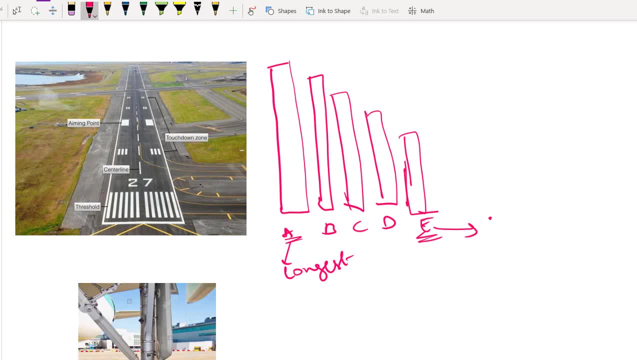 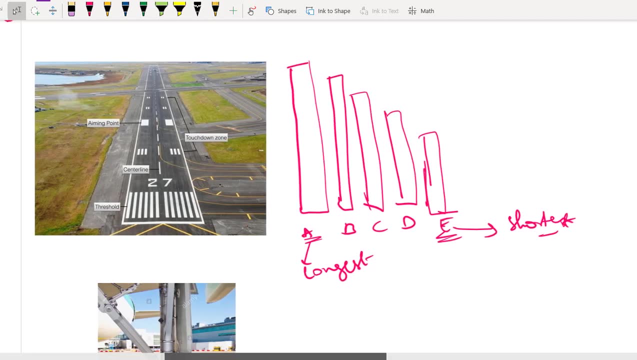 like that, so that you won't be having any confusion. A is the longest, E is the shortest runway. based on runway, we are classifying airports as airport A, airport B, airport C, airport D and airport E. now, similarly, based on equivalent single wheel load, we are classifying 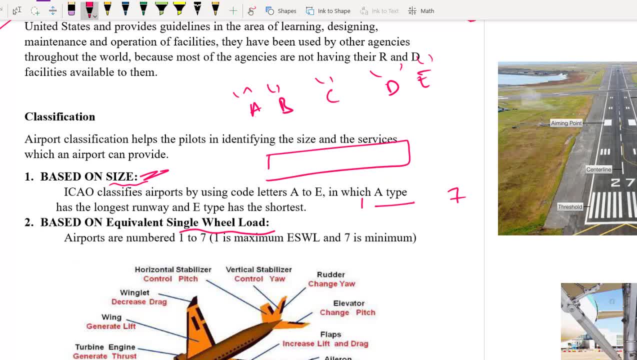 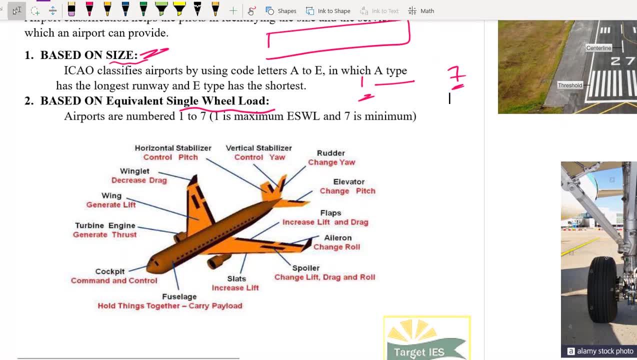 our airports as airport 1 to airport 7. airport 1 is very good, airport 7 is not so good. ok, so what is this equivalent single wheel load? if you are good at transportation, engineering one highway, if you have studied in your college, you must be knowing this equivalent single. 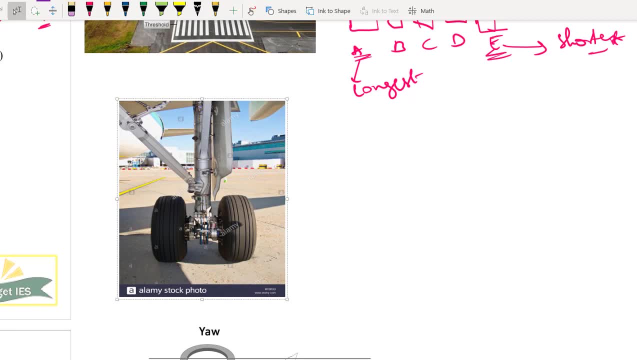 wheel load. but if you don't know, no issues, we will increase everything from scratch. see, basically leave this aircraft, because many of you might have not seen it, but you might have seen the buses right, you might have seen the trucks right. so, basically, how many types are there? there will be two. 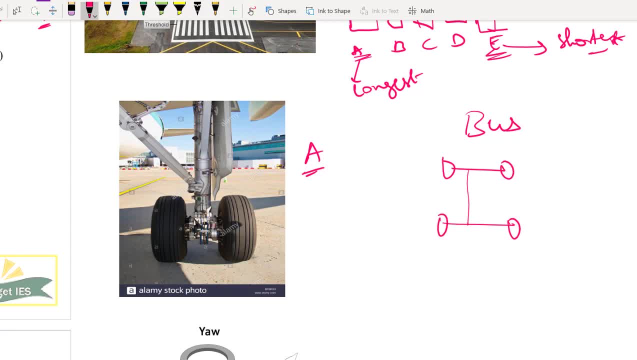 types here at front and there will be two types here at back right. so if you are taking a bus, there will be one, two, three, four, four types. but in some buses if the load is very high, you will be seeing there will be two more types here, agreed or not, one in return. 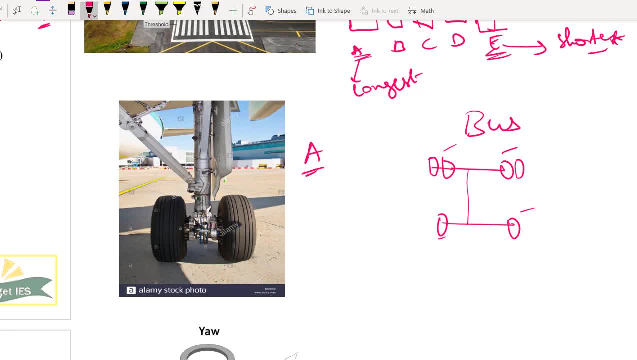 two will be there. if you are carrying super heavy loads, if you are going in like mining side where we use trucks, there will be even like four types here, right? so basically, how many types are there, even like four types here? surely you got the clarity right? so buses. 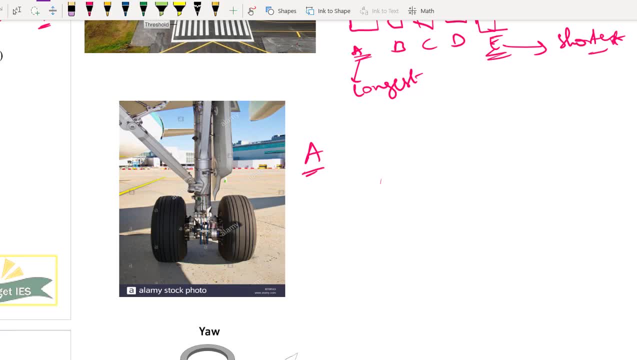 two types are very frequently seen in India, agreed or not. so what is happening? instead of one type, we are replacing with two types. right same concept is applied in the airport also. ok, if you have to carry a huge load. obviously, if we use two types, we will be going for four. 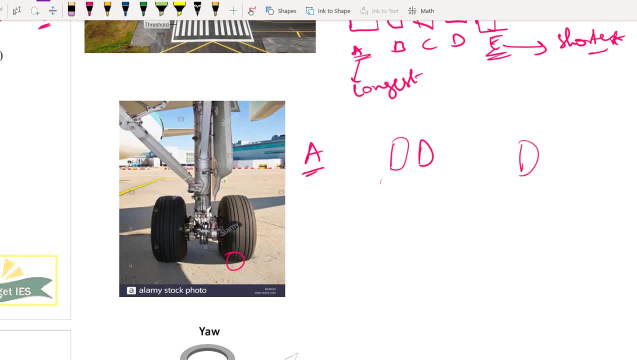 types. if you have a very big like air bus, you could even have six types or eight types. ok, how it will look if this is my airplane. right, let us say this is my airplane. you will be seeing only like here there will be two tires and here there will be one tire, three tires we basically see. 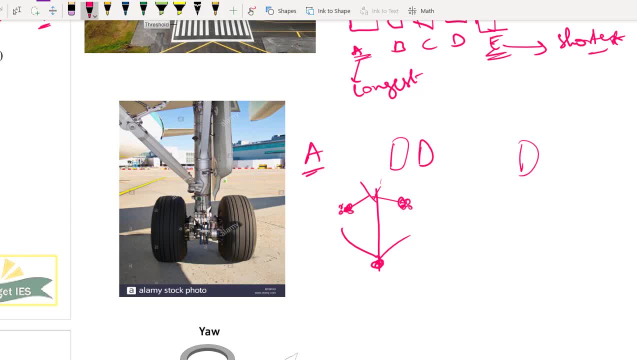 but here we will be having like two tires or four tires more than one in general. okay, i hope you got it right now. what is this equivalent? single wheel load. let us say there are two wheels, okay, and let us compare with single wheel. let us compare with single wheel. so if there is some vehicle which is 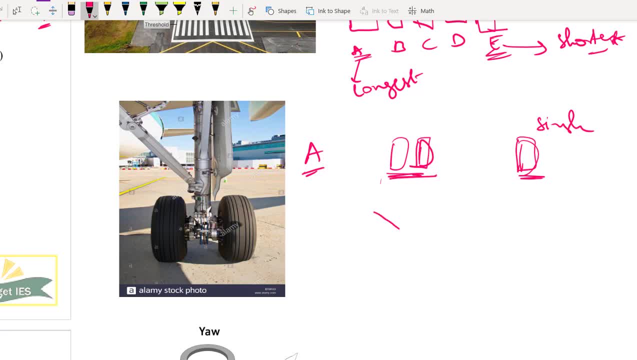 using two wheels instead of one wheel. obviously it will have certain amount of less deflection on the road right obviously whenever you are applying some load. so the deflection will be less, the stresses applied will be less, agreed stresses applied will be less and the contact pressure 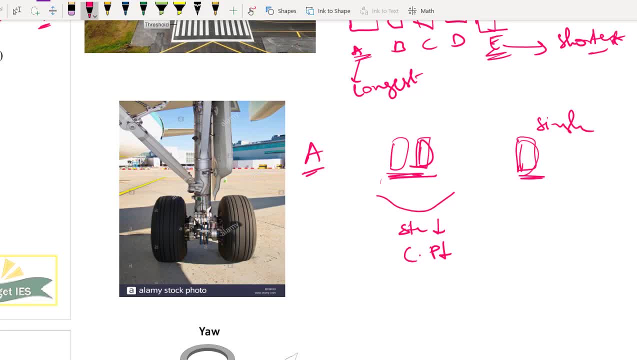 of these tires will also be less agreed or not. so, whatever this contact pressure or stresses being developed because of these two tires, if you are replacing by only one tire, okay, and whatever load you are applying to get the same voltage, you are applying to get the same voltage. you are. 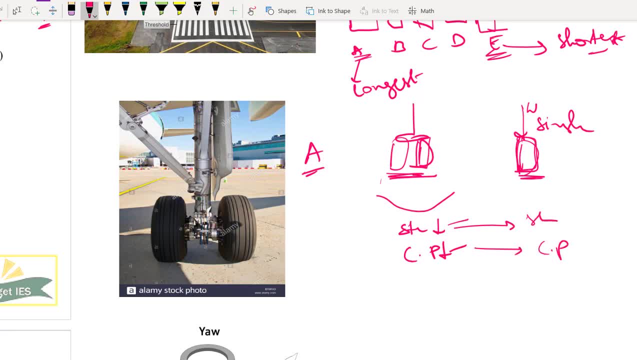 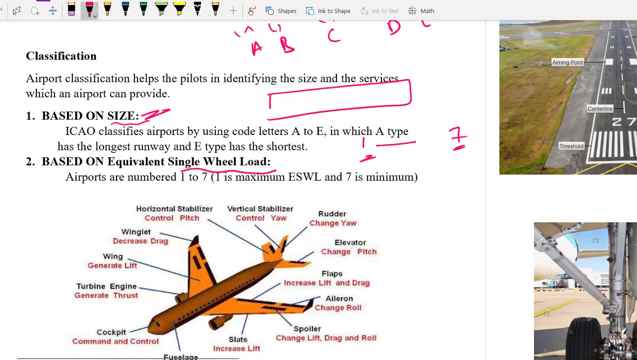 get the same amount of stress and same amount of contact pressure. we will be calling it as equivalent single wheel load. i hope concept is clear for you. so this equivalent single wheel load. based on that, we are again classifying our airports from one to seven group. one to group seven. 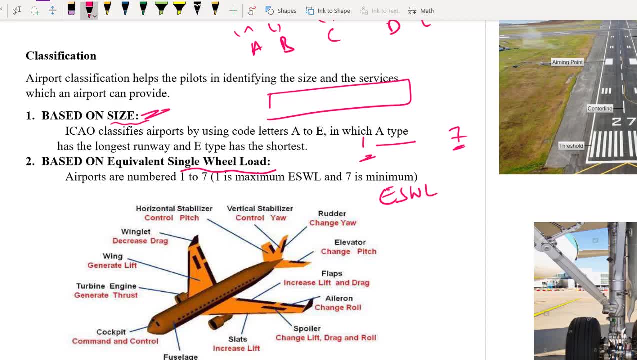 so one means it has a capacity to carry lot of equivalent single wheel load, which is very good, so it can take lot of weight without any problem. if you have a airport with grade seven, that means it cannot take that much amount of load on its runway. i hope concept is clear for you. 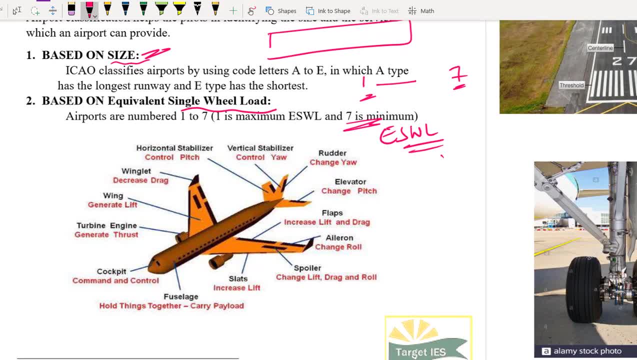 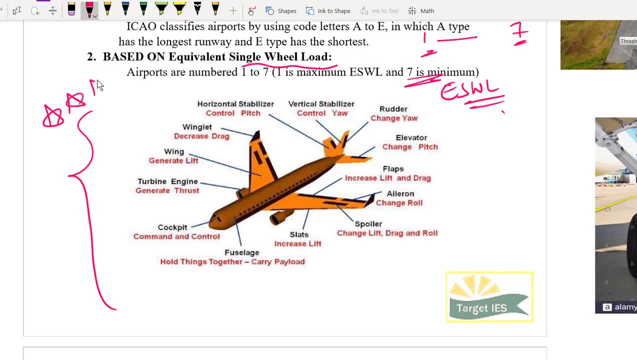 so this is about basics of classification of airport. now let us see some important parts of our aircraft, very important for one-liner examinations, like state psc- he could ask this as direct pits. so please do remember the first one is cockpit, so obviously you might be knowing. 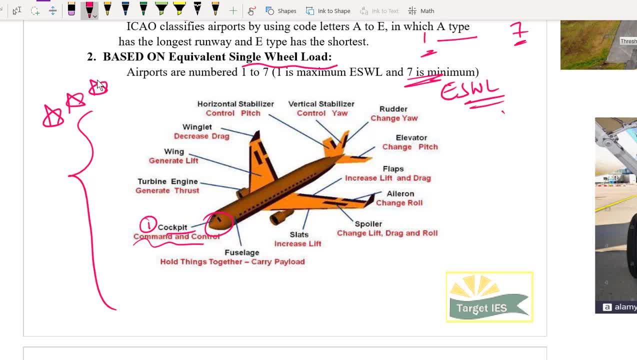 the cockpit right. this is the cockpit right. so, this is the cockpit right. this is the cockpit. this is where the pilot will sit and it is a command and control unit. okay, next is fuselage, the place where passengers sit right. we will be calling it as fuselage. it purpose is to carry. 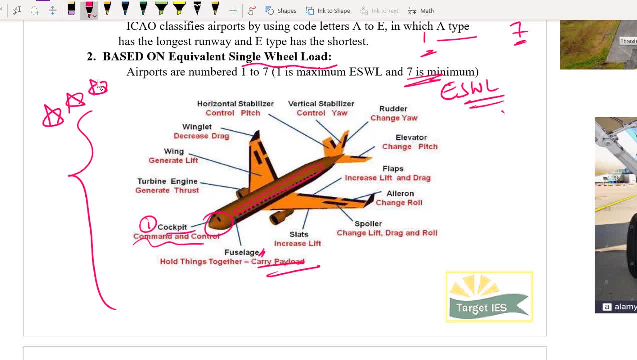 the payload. i hope it is. you are very clear. one: first is cockpit, next we have fuselage and obviously you will be having wings, you will be having turbine engines- basic term. but there are two very important things. one is rudder and elevator. please do remember rudder is used to 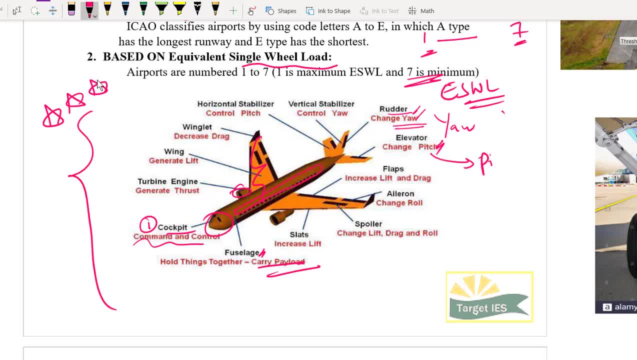 change yai and elevator is used to change yai and elevator is used to change yai and elevator is it is used to change pitch. now you can ask me, sir, what is yai and pitch? these are some basic terminology which you should know from your schools itself. but you don't know, no worries, i will teach. 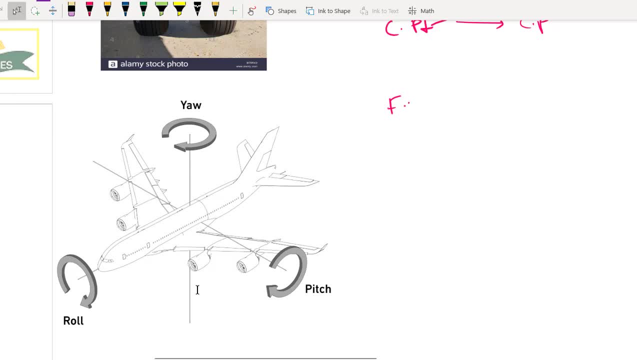 you again. okay, the same concept is applied in your fluid mechanics also. these terms do come in fluid mechanics also, like roll ho gaya, yai ho gaya and pitch ho gaya. okay, these are some important things which you have to understand. if you, the flight is rotating, we are talking about air. 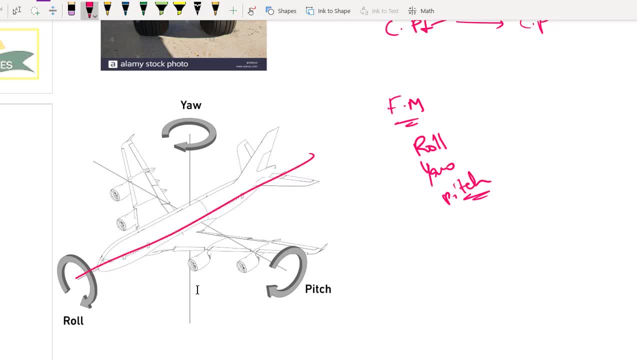 port. right, so let us talk about in the language of aircrafts: if my flight is rotating about my longitudinal axis, i will be calling it as rolling. okay, so if the flight is moving like this, like this or like this, we will be calling the flight is rolling, and next is pitch. what is pitching? see? 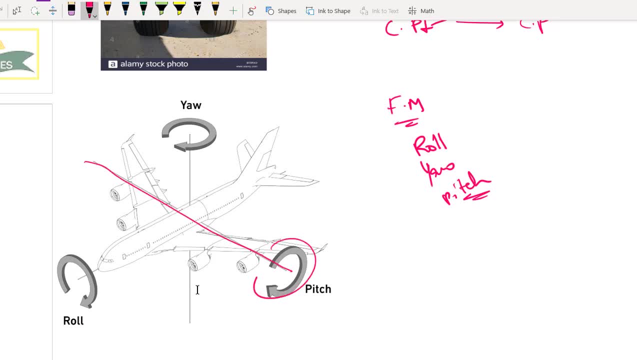 along the lateral axis. if there is any rotation, i will be calling it as pitching. i hope it is very clear right next, just draw a vertical line along this vertical axis. if it is revolving, then we will be calling it as yai. so to explain you, let us say: this is your human face, because we have a habit. 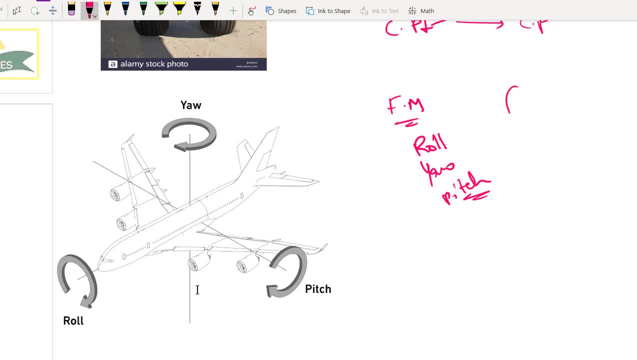 that we change the face very frequently. okay, so let us take this stickman face. okay, let us take this stickman face if you are saying yes. okay, when you say yes, what do you do, sir? you move up and down, up and down, right, so that will be nothing but pitch. okay, that will be nothing but pitch, please. 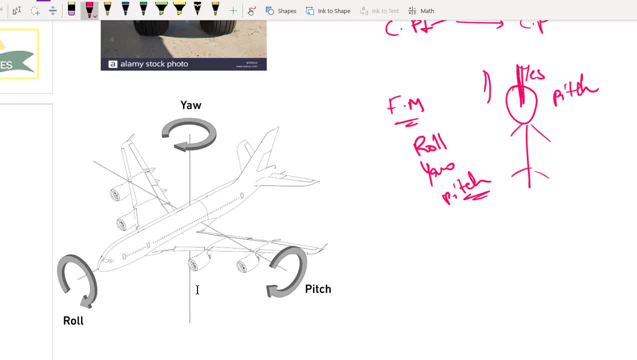 do imagine how you say yes, you will be lifting your face and, uh, moving it forward, right down, up and down. so that is pitching okay. along this axis you are rotating up and down, so it will be called as pitching okay. similarly, if you are saying no, if you are saying no, so obviously you will be moving. 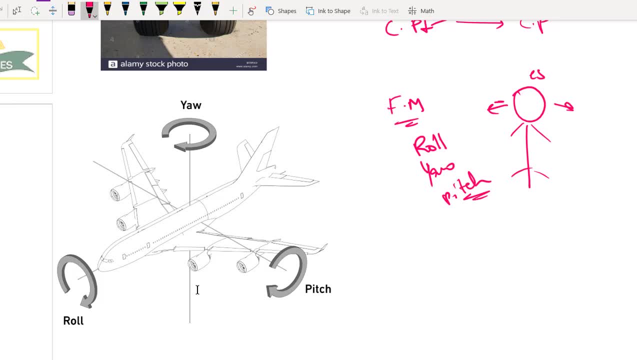 sideways, right. so this way, this way, you are saying sideways, that will be your yai, okay, that is your yai. so along this fixed axis, you are moving your head like this or like this. so that will be no, okay, no case. how do you do? you won't be moving your neck, just you will be moving your cheek. 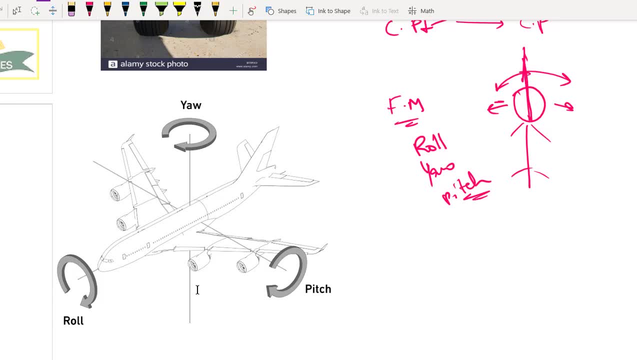 like this: right from left to right, left to right. so that is your yai along the vertical axis. if it is moving in these directions, then we will be calling it as yai. so now just imagine, this is your face right. so if you are rolling your face in this direction, if you are rolling your face in 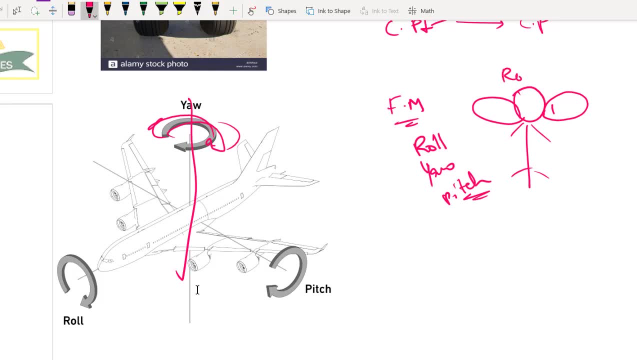 this direction. if you are moving your face like this, then that will be roll. i hope you got it right. you understood the application. now practice again. what is pitch? yes, just like how you say yes, sign language, okay, move your head up and down. that will be your pitch. similarly, flight be. 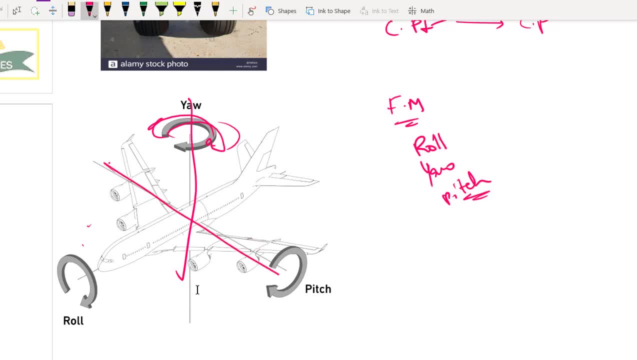 along this axis, you can imagine right. so this is happening. this part is going up and down, going up and down. okay, so next we have yai along the vertical plane. no, how do you say no, you will be moving the chin right. so if your flight is going like this or like this, then we will be. 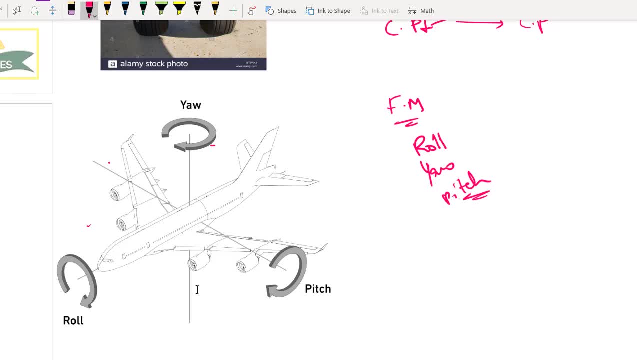 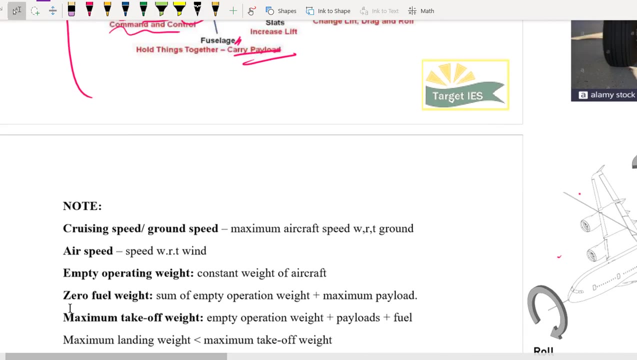 calling it as yai. okay, if the flight is rotating like this, okay, then we will be calling it as roll along the longitudinal axis. okay, i hope you got it right. you understood pitch, yai, and rolling. so to control this, yai, we have a instrument called as rudder. give it. 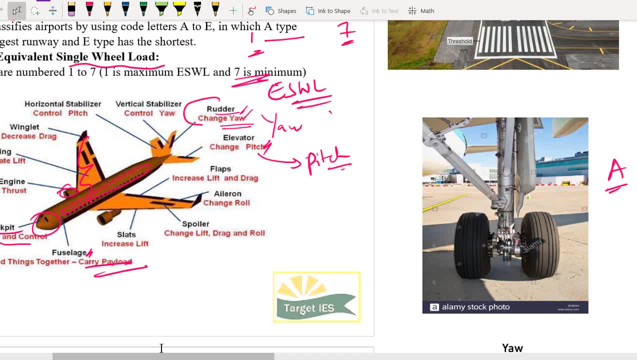 five star very frequently ask it: wait, what is rudder? it is used to change yai, and what is elevator? it is used to change the pitch. if this pitch is this elevator, it will not allow my flight- whatever, it was something like this right, it will not allow it to rise like this, okay, like this, okay. 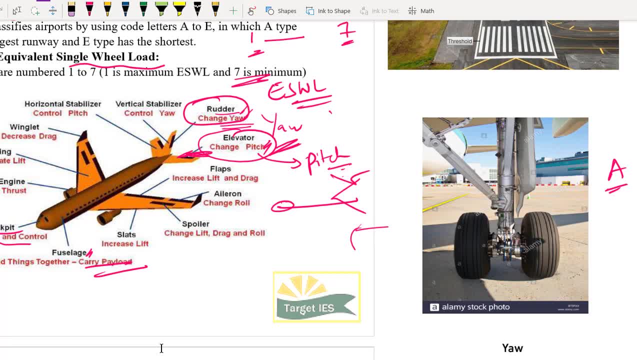 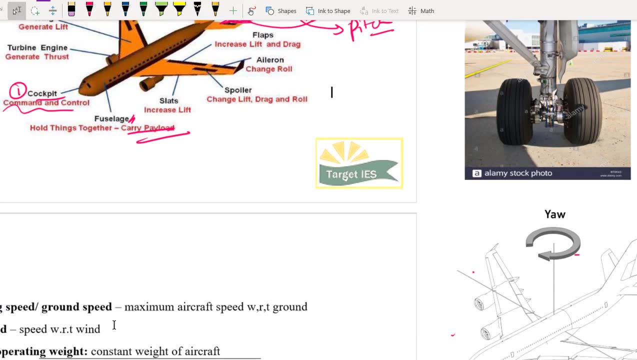 it will not allow it to shift. it will maintain its elevation in whatever position you want. i hope it is very clear for you, right? so two very important things: rudder and elevator frequently ask it bits so remaining. you can obviously answer like wing or turbine engine. obviously you can. 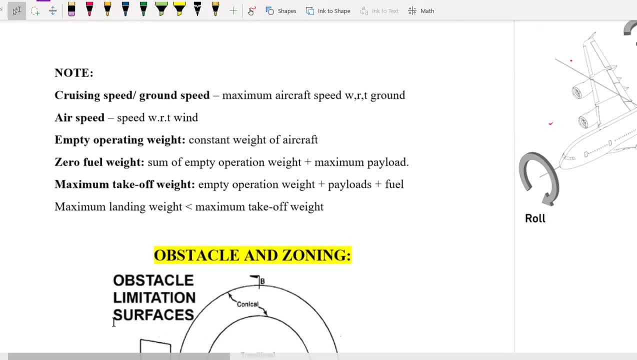 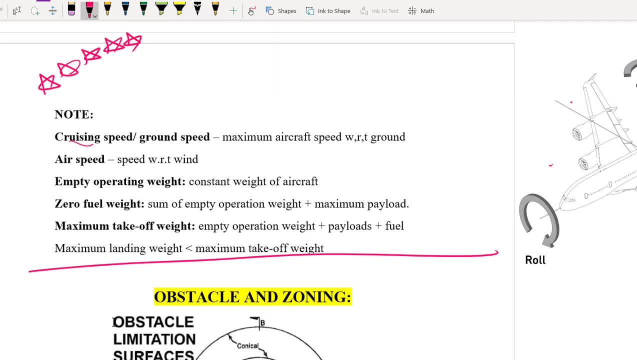 answer: not a big deal. so there are few more terminologies and after that i will stop. very important, give it five star again. okay, super important thing. so first one is cruising speed. whenever i am talking about cruising speed of aircraft, i am talking about its speed relative to the ground surface. okay, when i am talking about 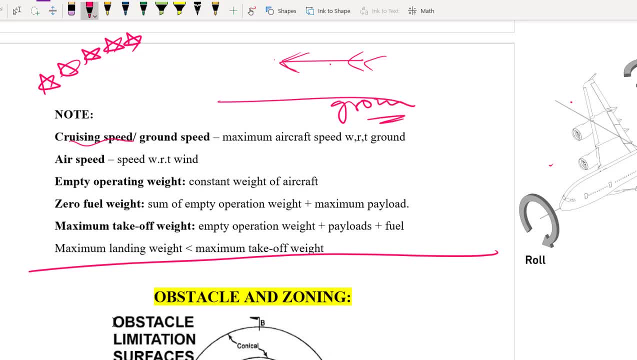 ground speed or cruising speed. i am talking the aircraft speed with respect to my ground surface. next is airspeed. obviously you can understand right: aircraft speed with respect to air. i will be calling it as airspeed. next is empty operation weight- very important. these three empty operation weight, see, it is the constant weight of your aircraft. so if this is your, 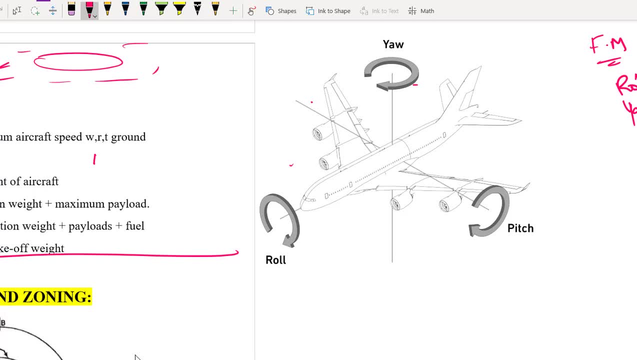 aircraft. the constant weight, whatever you are talking about, it is the airspeed of the aircraft- is there, which will be always constant. okay, if there are no people, even then it will be constant. if there is no pilot, even then it will be constant. if there is no fuel, even it will be constant, right, 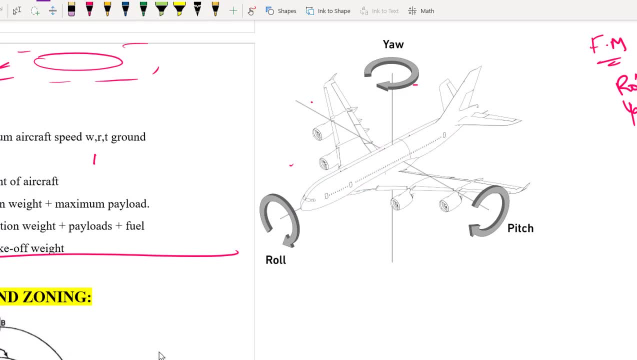 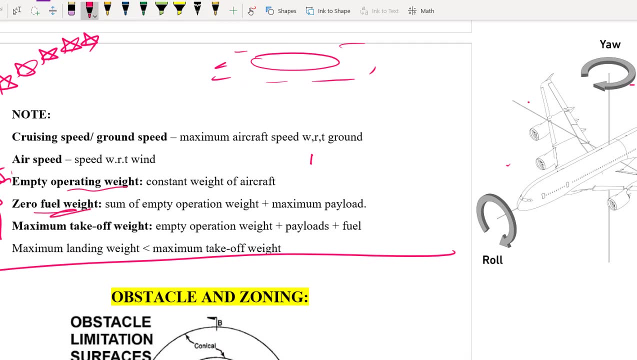 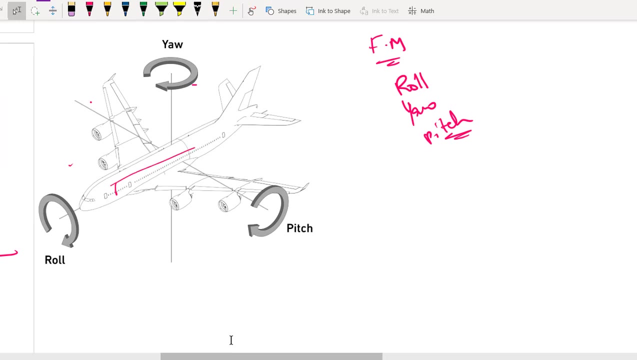 it is just frame kvgs and there's a furniture. so this all is included in your empty operation weight. i hope it is very clear. right next is zero fuel weight. zero fuel weight sum of empty operation weight plus maximum payload. so maximum payload means it could be passengers or cargo. okay.